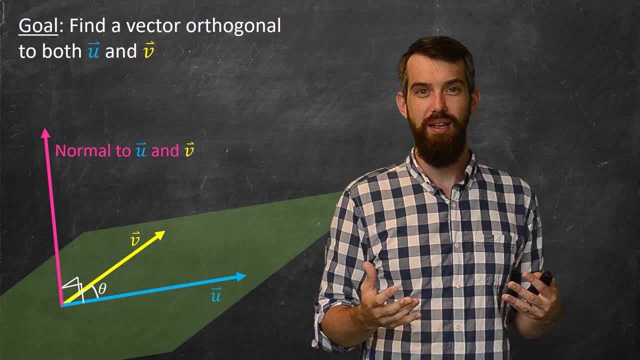 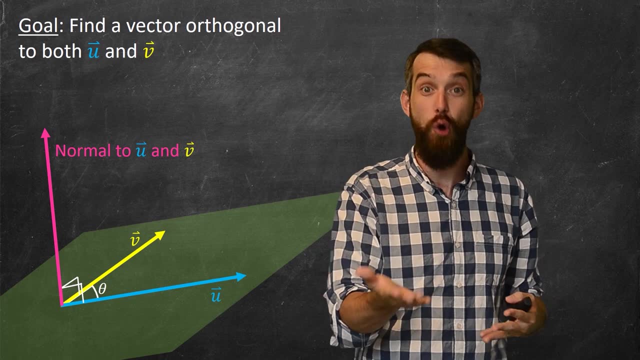 looking for a normal vector that looks something like this. The idea is that when you have some plane- the way it tilts and is oriented in three dimensions- you can get this information out of the normal vector, And hence we're interested in the normal. 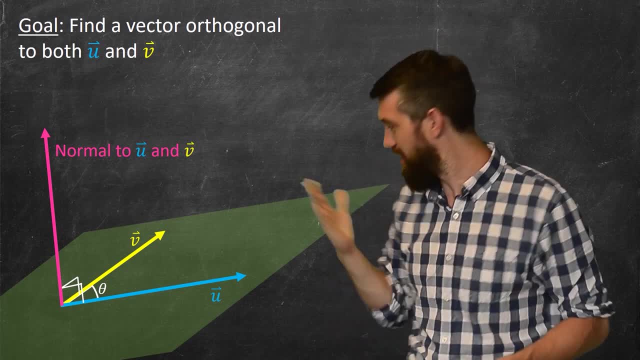 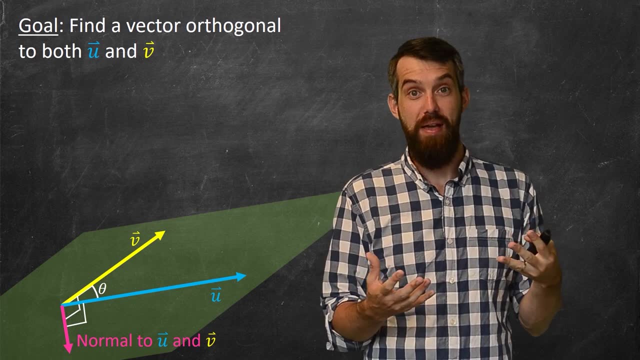 vector. Now, the problem is there isn't one normal vector. This is a normal vector, but this little short one which is pointing down underneath the plane is also a normal vector And indeed, multiplying by any non-zero scalar is going to give another perfectly reasonable normal for this. 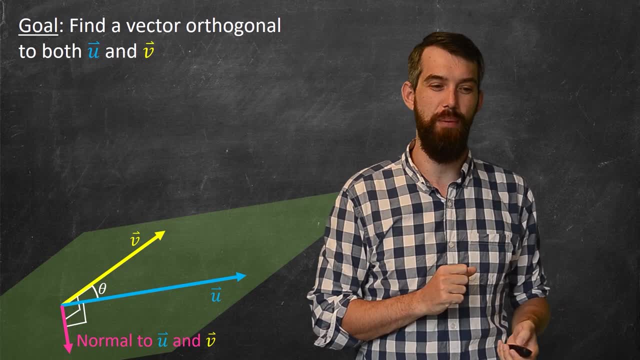 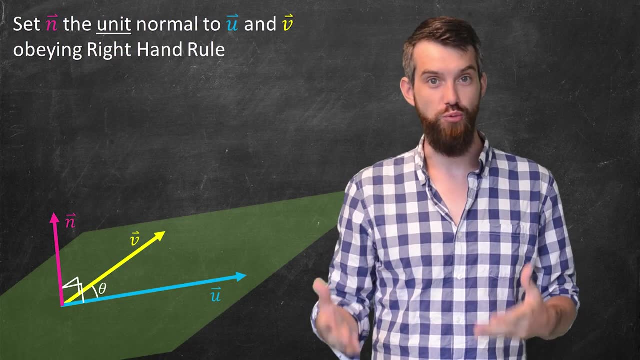 purpose. So that's fine, but I'm going to choose one in particular. I'm going to choose the so-called unit normal that obeys the right-hand rule. The way the right-hand rule works is that when you take your right hand- because it's called the right-hand rule- and first of all you point it, 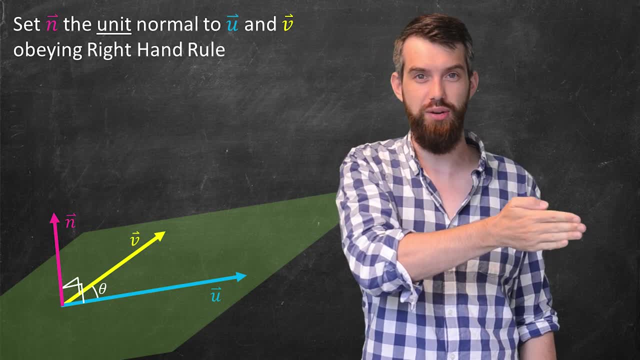 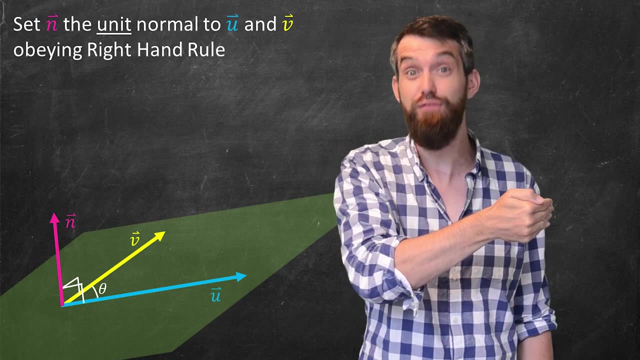 along the direction of the u vector, the first vector that you're considering. So your finger's pointing in the direction of the first vector, And then what they do is they curl towards the second vector, to the v vector. in this case, They point along u and they curl to v. And then, if you 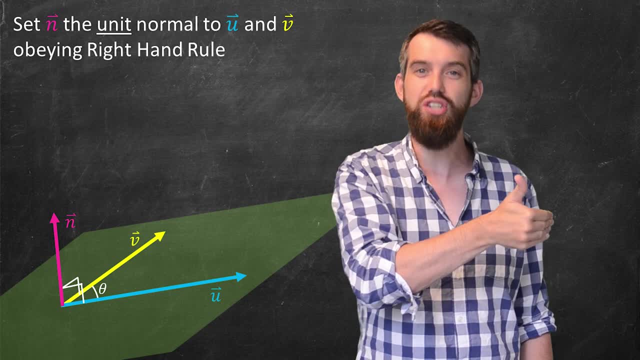 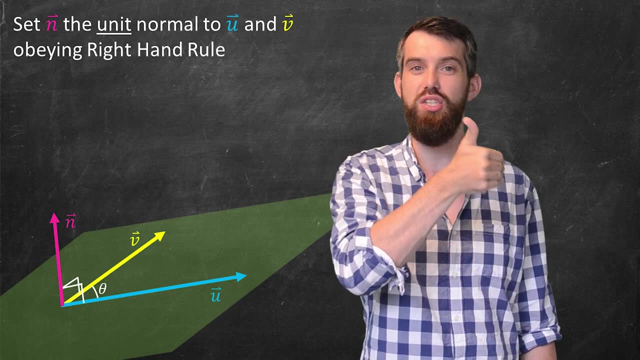 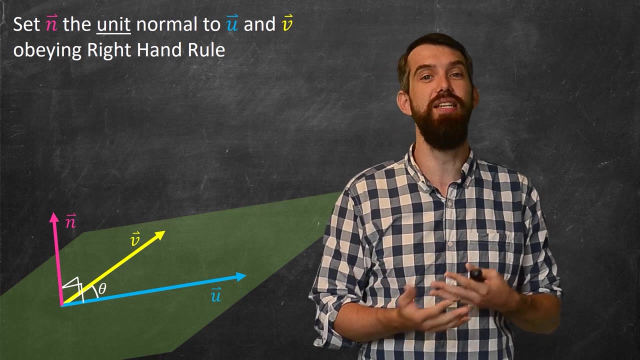 stick your thumb up. your thumb is going to tell you the direction of the normal that we're talking about, And it curls up to become this normal, which is upwards in our case. If I only demanded that it was a unit vector, there was the two: one pointing up, one pointing down. When you say it's, 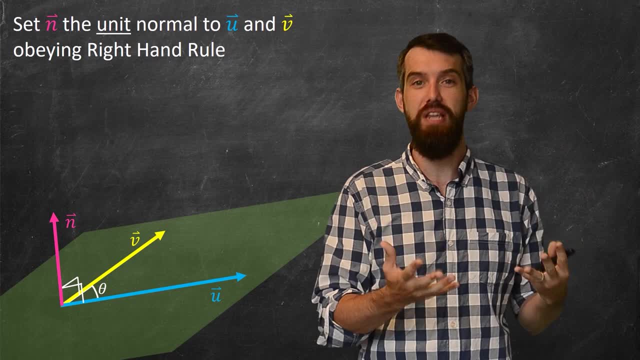 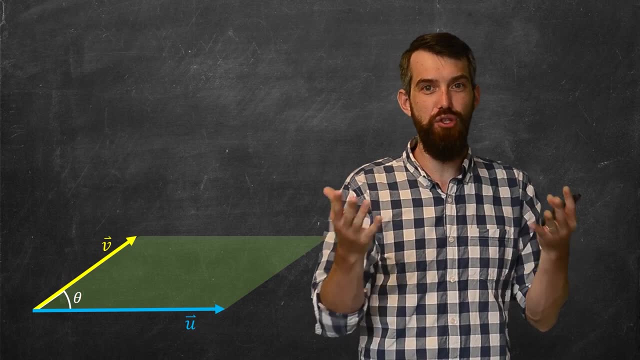 the one vector prescribed by the right-hand rule. it tells you there's only one unique vector that obeys these properties. So that was one geometric problem. but I'm going to tell you about a different one. If I take those two vectors, remember before we'd had a whole plane that 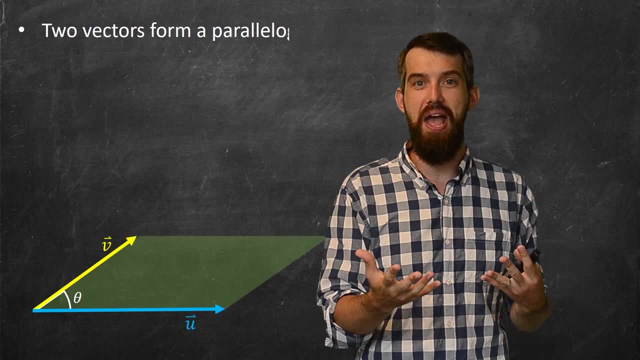 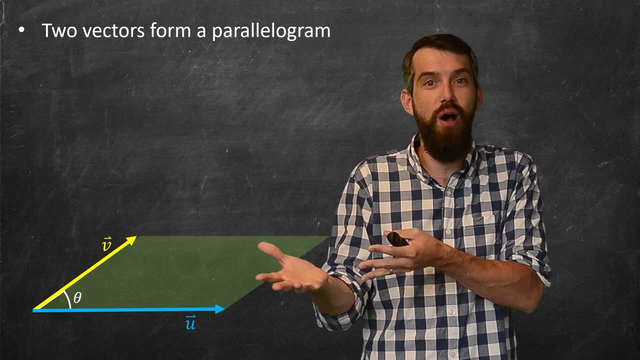 was spanned, but I want to restrict myself to the parallelogram that is formed by these two different vectors. It's got the vectors u and v on the one side, and indeed u and v on the other sides as well when you translate them around. 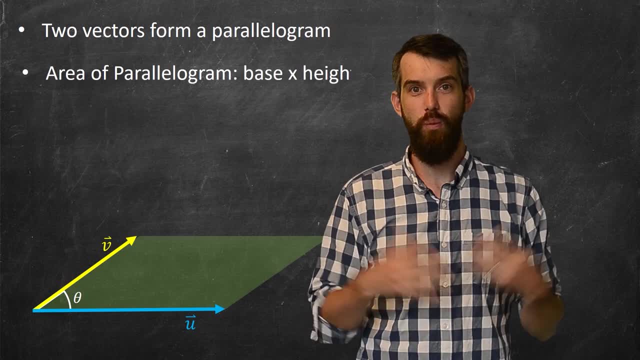 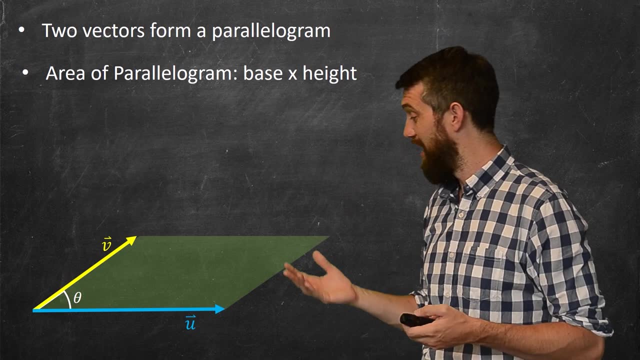 So the other question is: what is the area of this parallelogram? Well, the formula for the area of a parallelogram is base times height. Indeed, to see this, you can sort of see that there's. it looks like a parallelogram, but if I take this triangle on the one side, I can sort of put it on the other. 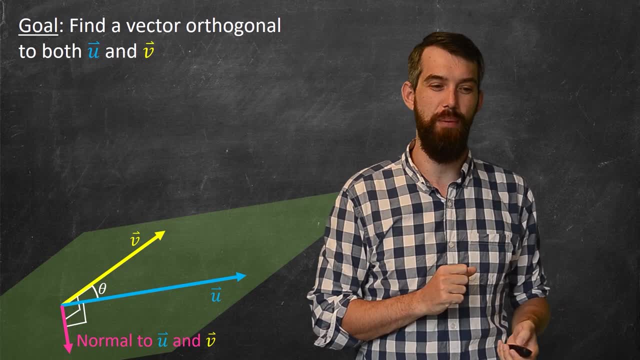 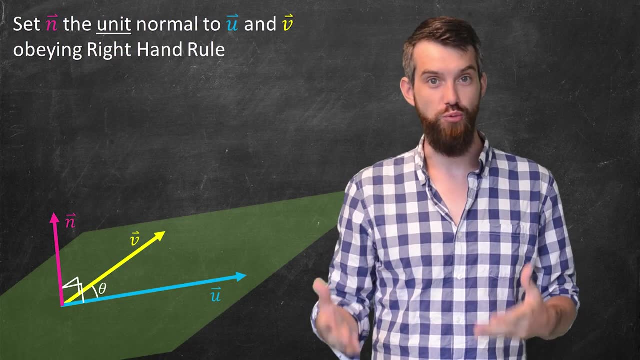 purpose. So that's fine, but I'm going to choose one in particular. I'm going to choose the so-called unit normal that obeys the right-hand rule. The way the right-hand rule works is that when you take your right hand- because it's called the right-hand rule- and first of all you point it, 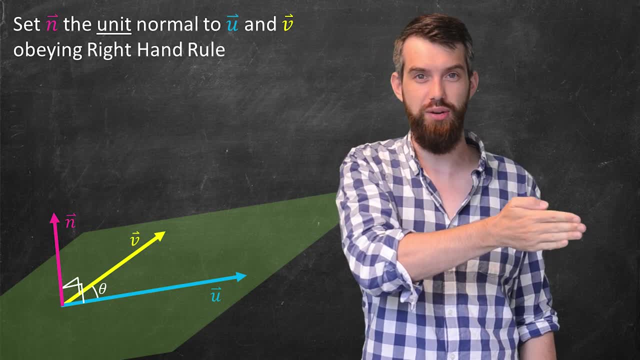 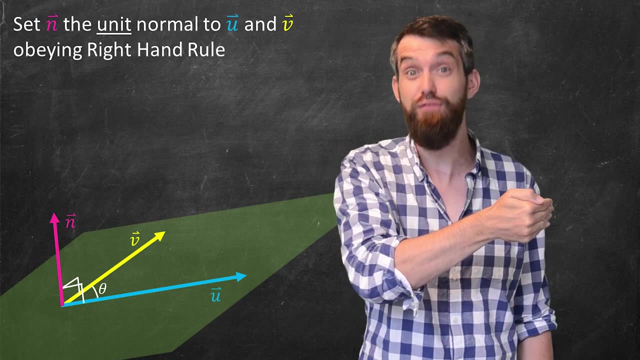 along the direction of the u vector, the first vector that you're considering. So your finger's pointing in the direction of the first vector, And then what they do is they curl towards the second vector, to the v vector. in this case, They point along u and they curl to v. And then, if you 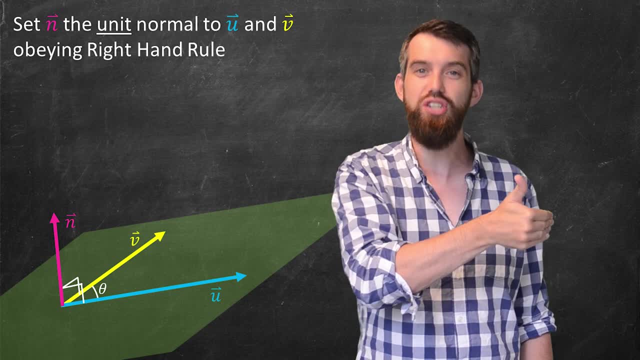 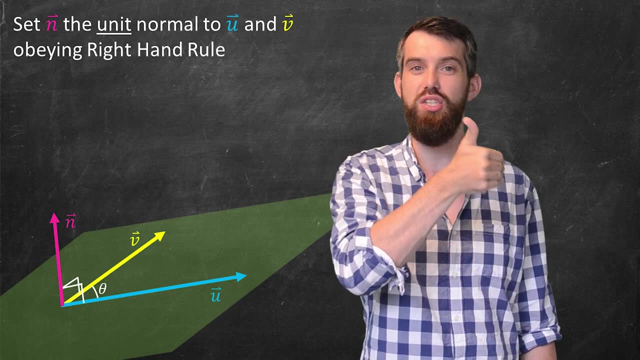 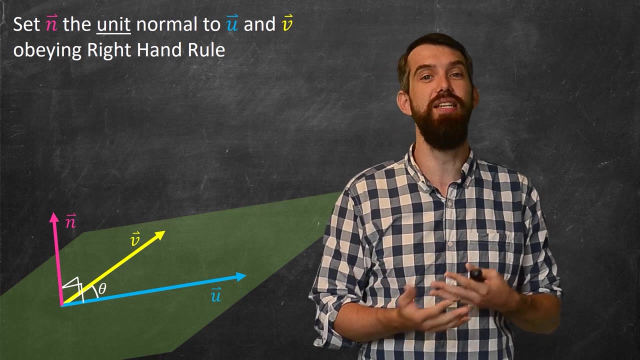 stick your thumb up. your thumb is going to tell you the direction of the normal that we're talking about, And it curls up to become this normal, which is upwards in our case. If I only demanded that it was a unit vector, there was the two: one pointing up, one pointing down. When you say it's, 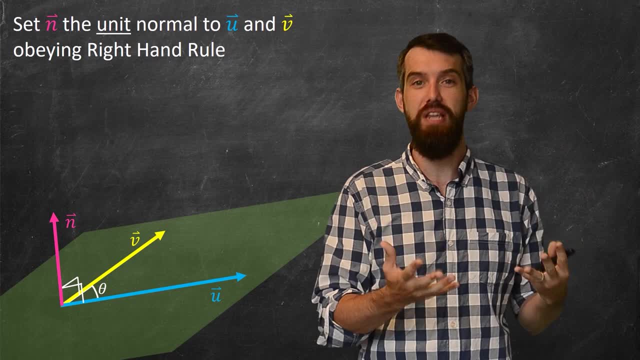 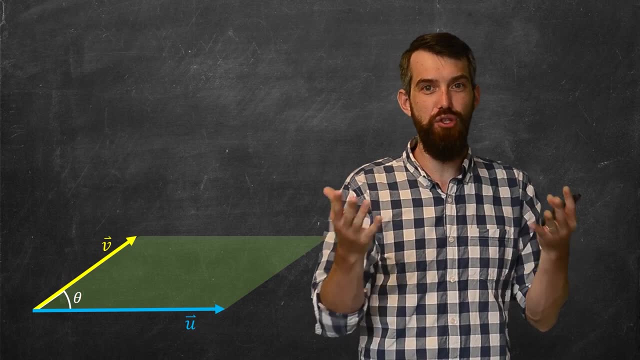 the one vector prescribed by the right-hand rule. it tells you there's only one unique vector that obeys these properties. So that was one geometric problem. but I'm going to tell you about a different one. If I take those two vectors, remember before we'd had a whole plane that 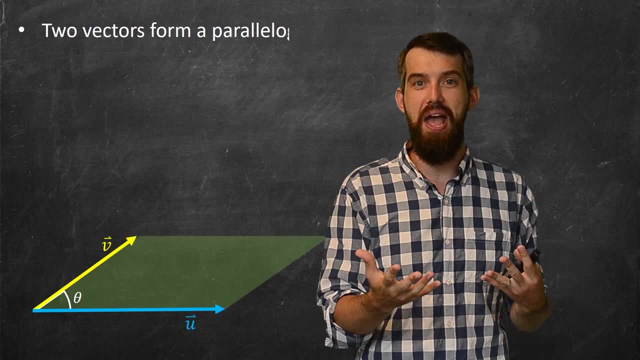 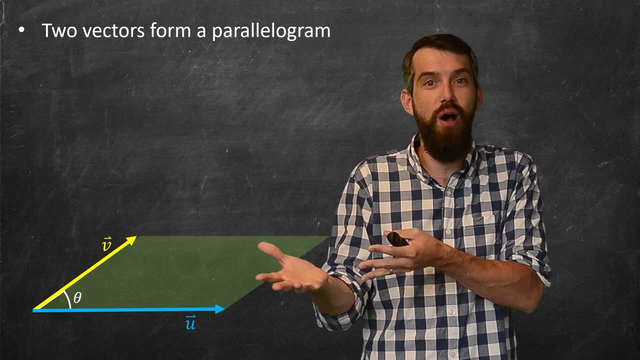 was spanned, but I want to restrict myself to the parallelogram that is formed by these two different vectors. It's got the vectors u and v on the one side, and indeed u and v on the other sides as well when you translate them around. 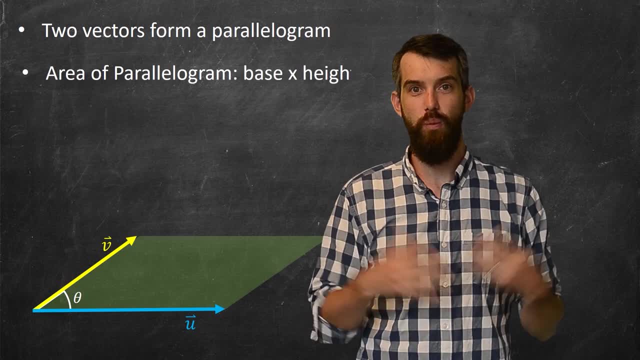 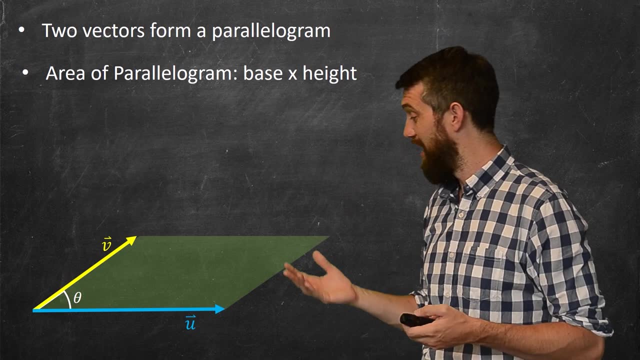 So the other question is: what is the area of this parallelogram? Well, the formula for the area of a parallelogram is base times height. Indeed, to see this, you can sort of see that there's. it looks like a parallelogram, but if I take this triangle on the one side, I can sort of put it on the other. 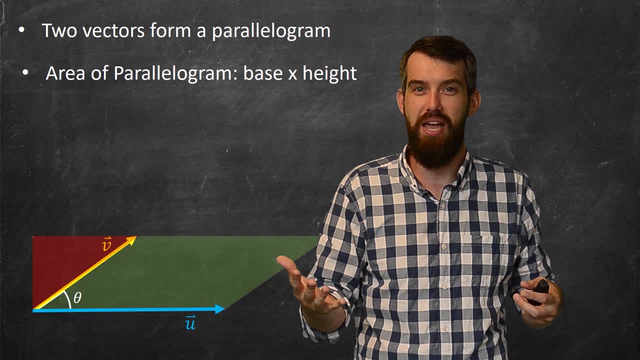 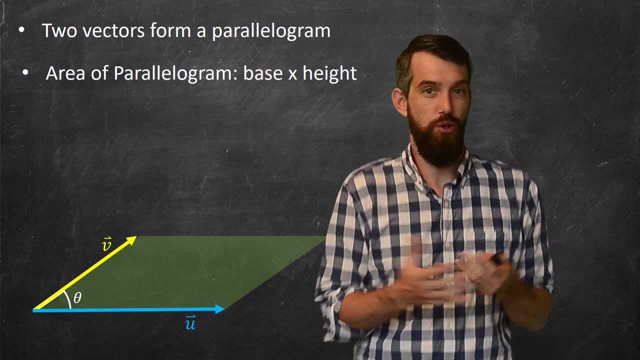 side and that would form a rectangle, and rectangle is base times height. So, nevertheless, the area of the parallelogram is base times height. But what's the height of this thing? I have this value theta, so I know what the height is. is going to be the length of v, sine theta, with a little bit of. 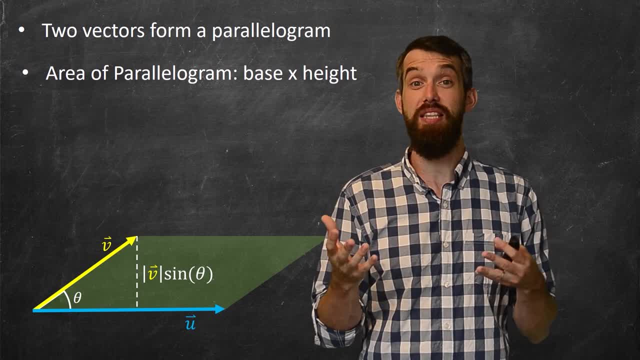 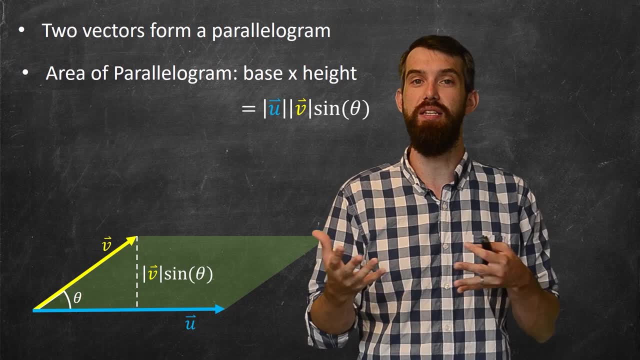 trigonometry on that triangle. All right, so then, what is the area of the parallelogram? It's the base times height. so the length of u is the base multiplied by this height, so the length of u, the length of v, sine theta. Okay, so I'm going to put these two different problems together of. 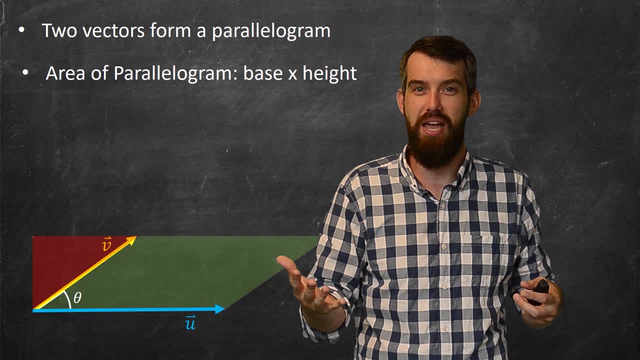 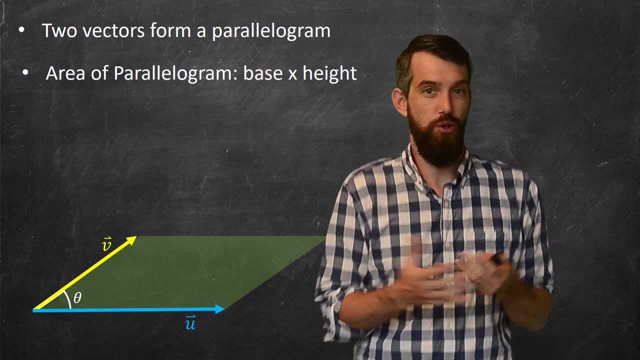 side and that would form a rectangle, and rectangle is base times height. So, nevertheless, the area of the parallelogram is base times height. But what's the height of this thing? I have this value theta, so I know what the height is. It's going to be the length of v, sine theta, with a little bit of. 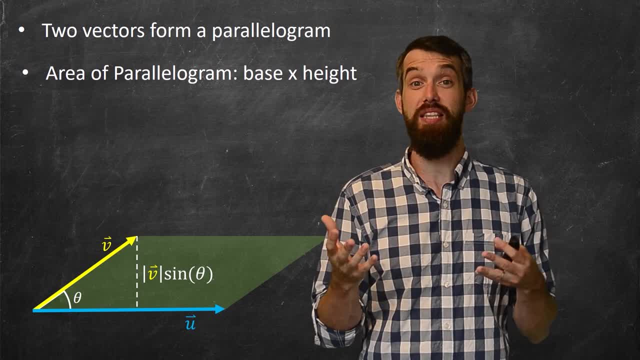 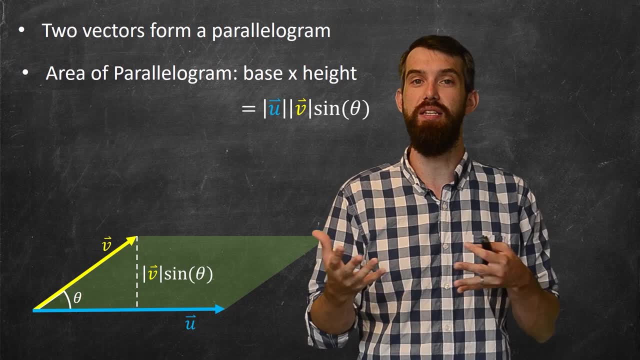 trigonometry on that triangle. All right, so then, what is the area of the parallelogram? It's the base times height. so the length of u is the base multiplied by this height, so the length of u, the length of v, sine theta. Okay, so I'm going to put these two different problems together of. 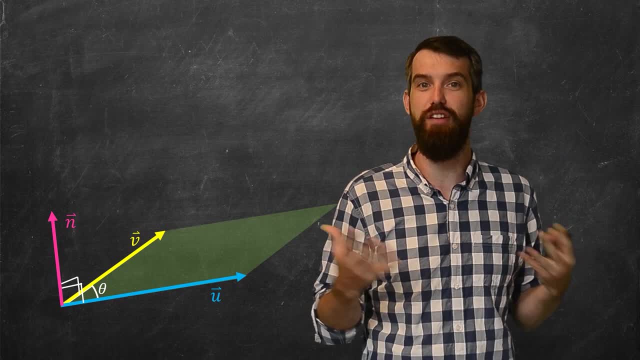 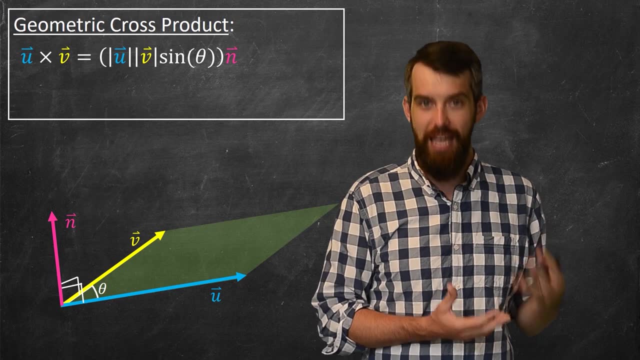 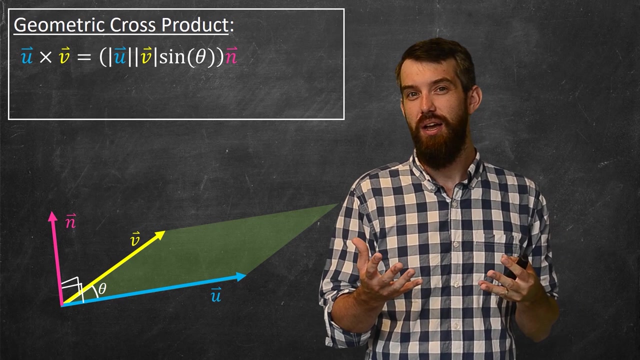 finding a normal vector to a plane as well as the area of a parallelogram, and thus I'm going to define my geometric cross product to be that the cross product of u and v is the vector that is in the direction of the unit normal, the m vector, but whose length 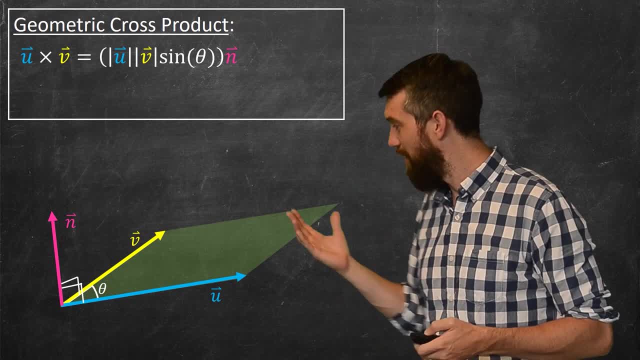 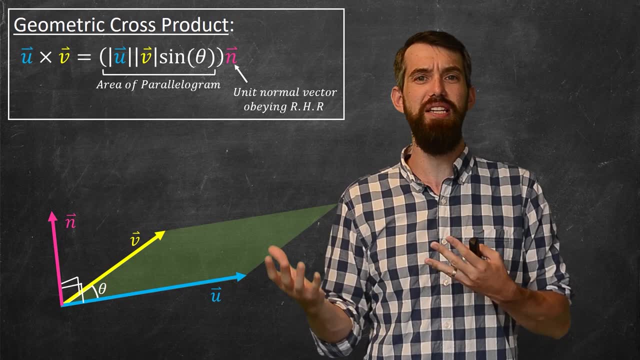 the scalar multiple is the area of the parallelogram. Namely, it's the area of the parallelogram multiplied by that unit, normal obeying the right-hand rule. This is very convenient. This cross product, we've defined this way, solves both of these different problems. 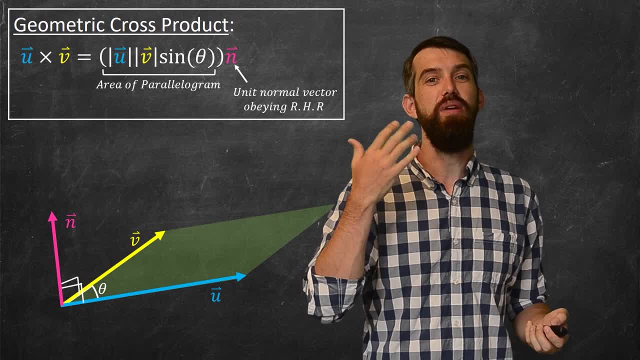 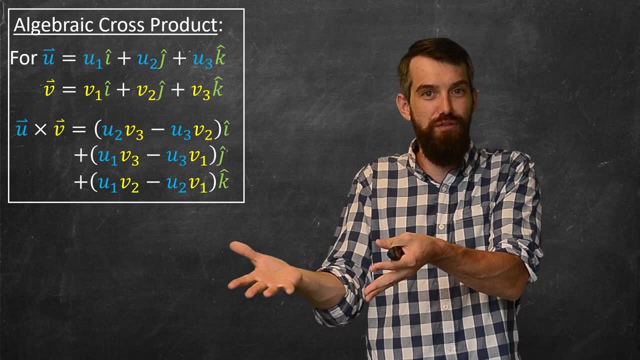 but how do you compute it? Now I'm going to put up on the screen the geometric cross product and it gives an answer for some easy-to-compute thing that just spits out the numbers, if you know what the u and what the v are. What I haven't justified and I'm not going to do in this 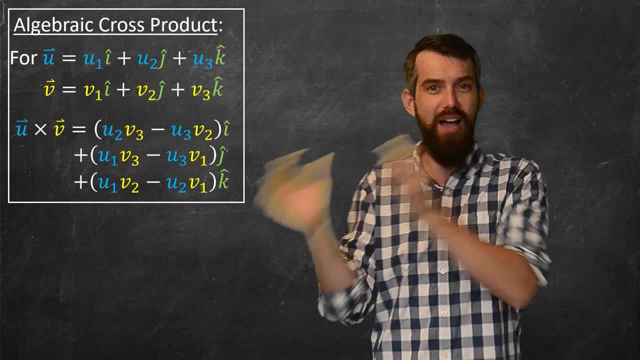 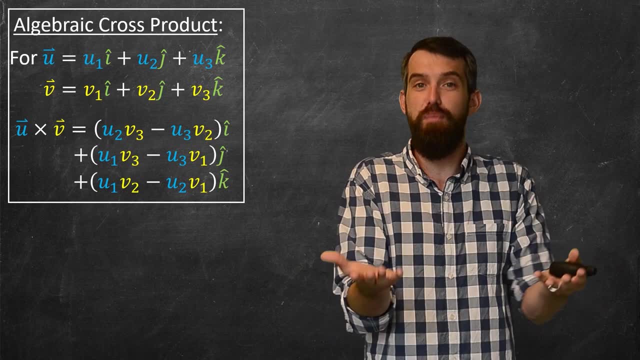 particular video is the connection? Why is the geometric and the algebraic versions of this cross product really the same? They are connected and you can show this, But nevertheless, for the purposes of this video, if you want to compute that cross product that we've seen before, well, 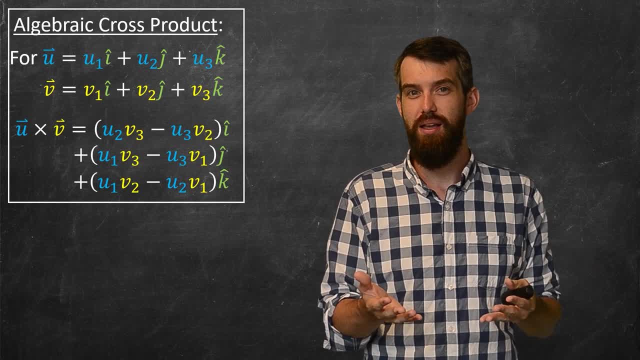 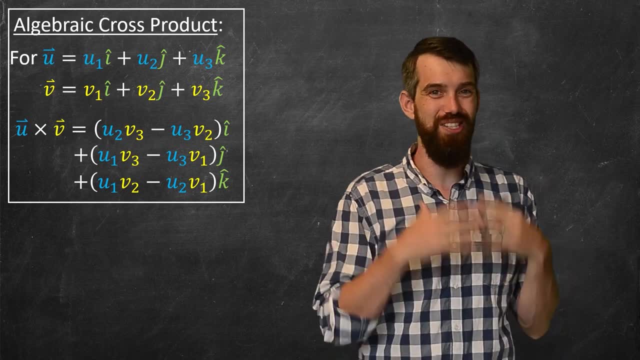 just plug it into that formula. It looks a little bit messy. And then the final thing I'll note is that if you've seen linear algebra before, if you've seen linear algebra before, if you've seen idea of a determinant, this messy formula that I don't really like, well, you can clean it up a. 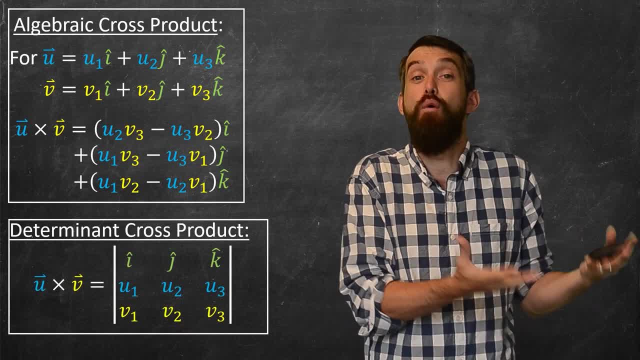 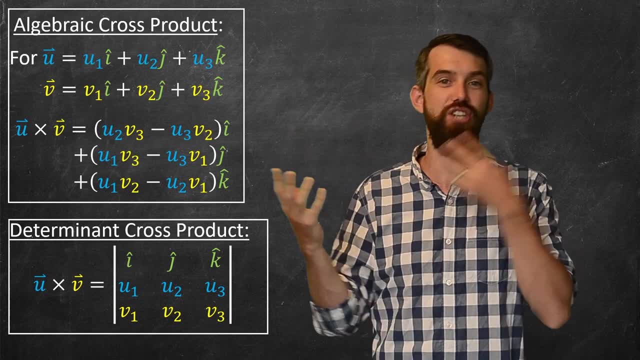 little bit with a determinant. The determinant form of the cross product is that the cross product of u and v is just going to be well, in the top row of your matrix you write i, j, k, then u1, u2, u3 in the next row and v1, v2, v3 in the final row, and then you take the. 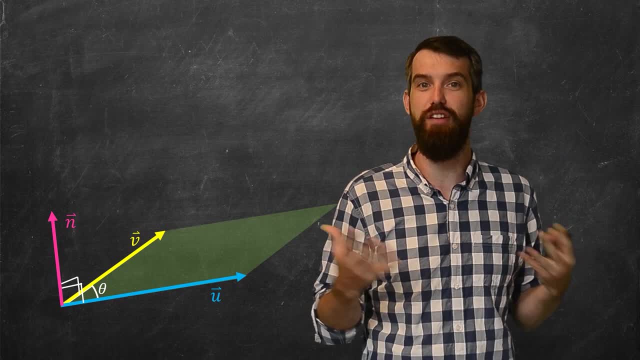 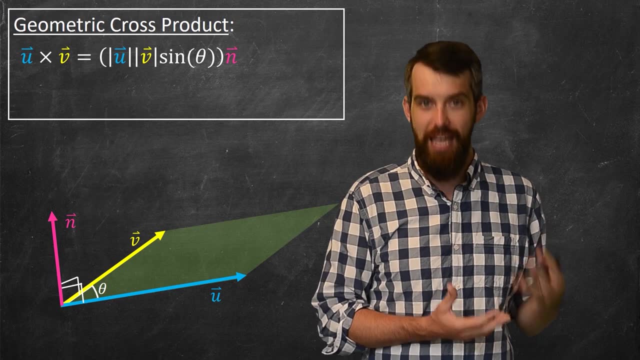 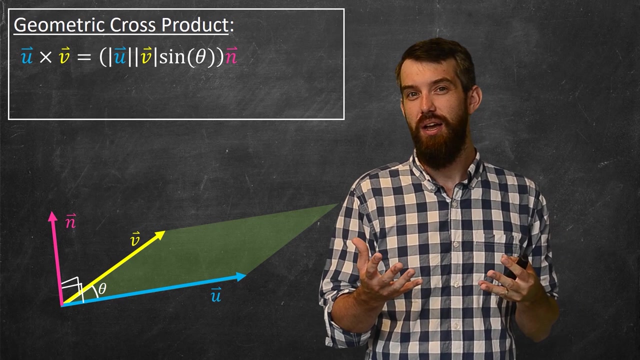 finding a normal vector to a plane as well as the area of a parallelogram, and thus I'm going to define my geometric cross product to be that the cross product of u and v is the vector that is in the direction of the unit normal, the m vector, but whose length 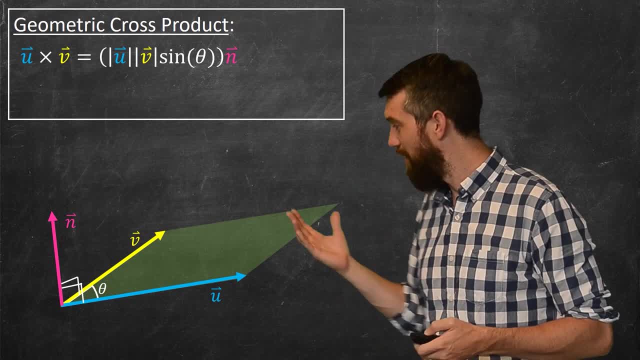 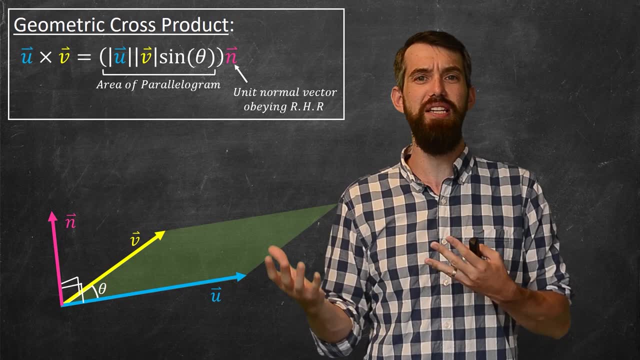 the scalar multiple is the area of the parallelogram, namely it's the area of the parallelogram multiplied by that unit, normal obeying the right-hand rule. This is very convenient. this cross product, we've defined this way, solves both of these different problems. 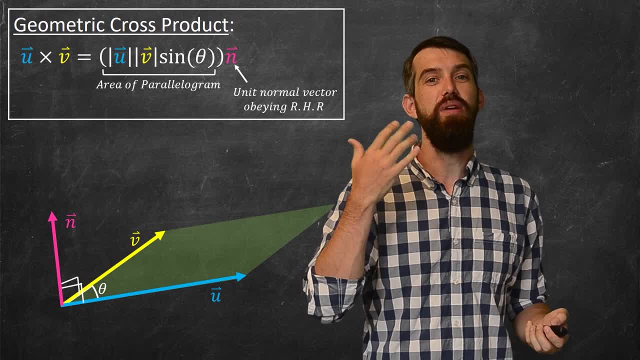 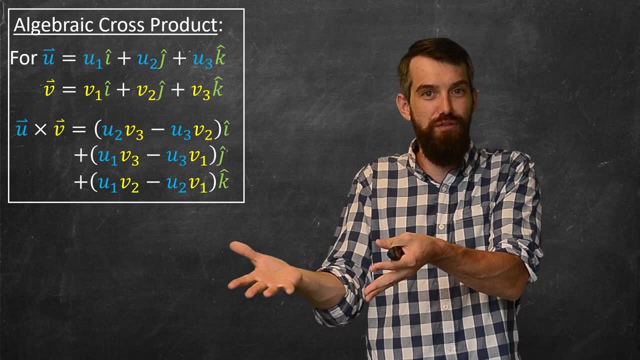 but how do you compute it? Now I'm going to put up on the screen the geometric cross product and it gives an answer for some easy to compute thing that just spits out the numbers, if you know what the u and what the v are. What I haven't justified and I'm not going to do in this 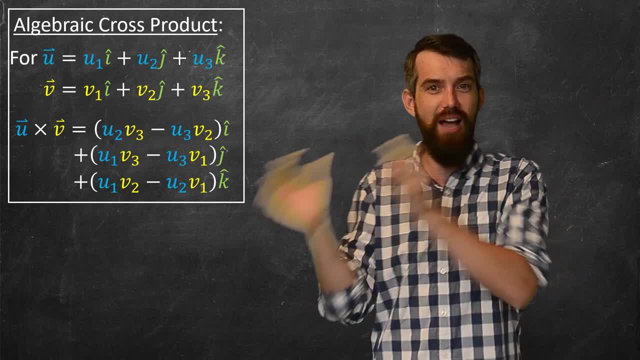 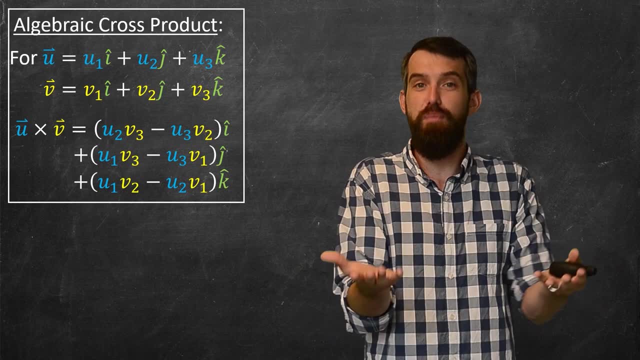 particular video. is the connection? Why is the geometric and the algebraic versions of this cross product really the same? They are connected. you can show this, But nevertheless, for the purposes of this video, if you want to compute that cross product that we've seen before, well, just plug it. 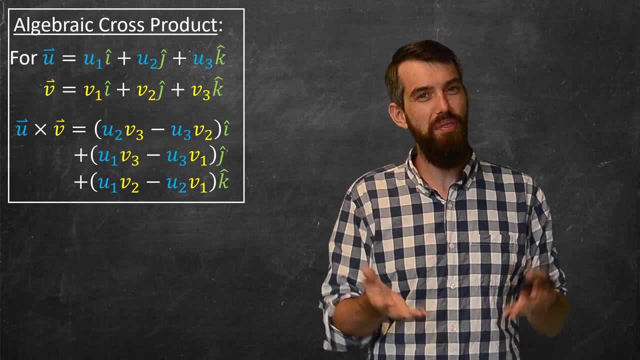 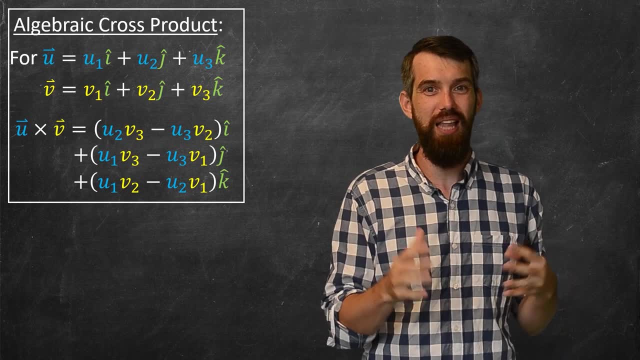 into that formula. it looks a little bit messy. And then the final thing I'll note is that if you've seen linear algebra before, if you've seen idea of a determinant, this messy formula that I don't really like, well, you can clean it up a. 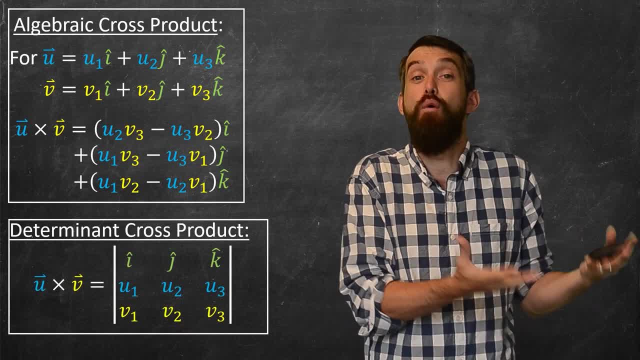 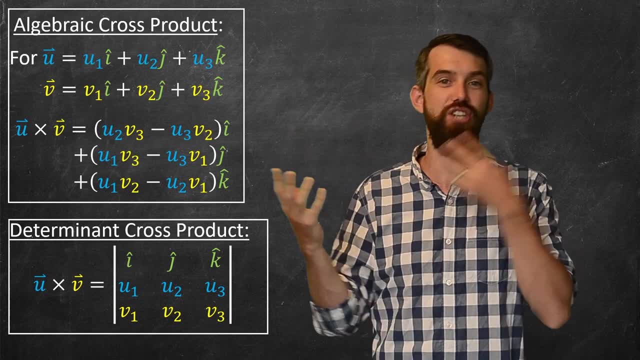 little bit with a determinant. The determinant form of the cross product is that the cross product of u and v is just going to be well, in the top row of your matrix you write i, j, k, then u1, u2, u3 in the next row and v1, v2, v3 in the final row, and then you take the. 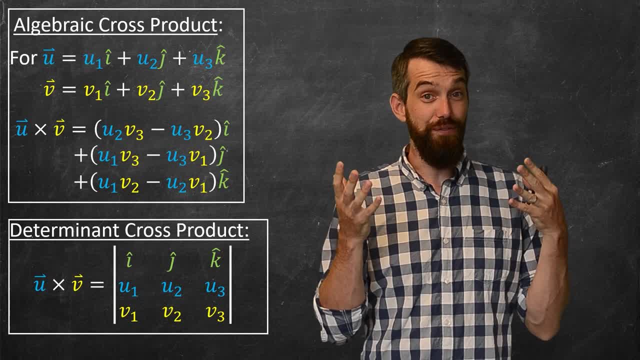 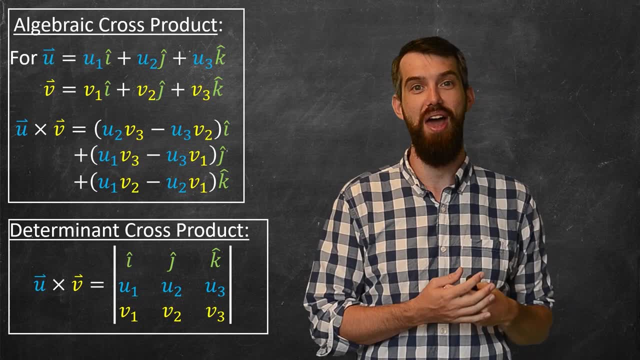 determinant of that. If you don't know what a determinant is, that is fine. you can either go and look it up for your identification or you can just always use the determinant. I'm going to use the top box, the version that just tells you how to memorize all that annoying. 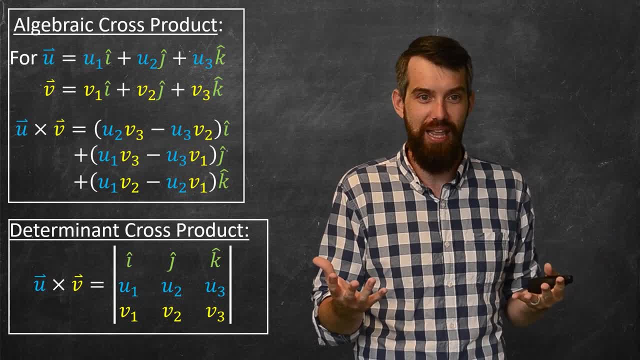 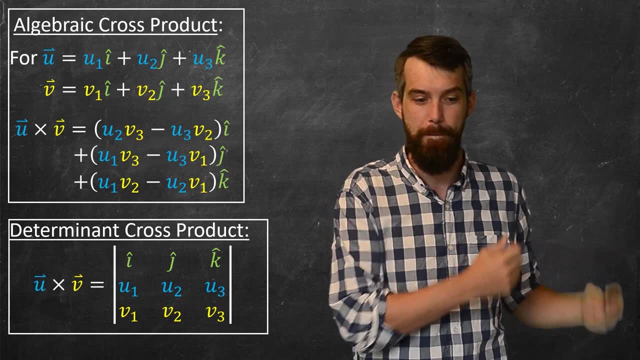 stuff. The determinant just gives a slightly easier way to memorize it. Nevertheless, we have an algebraic computation we can do. that corresponds to that geometric idea we introduced at the beginning.